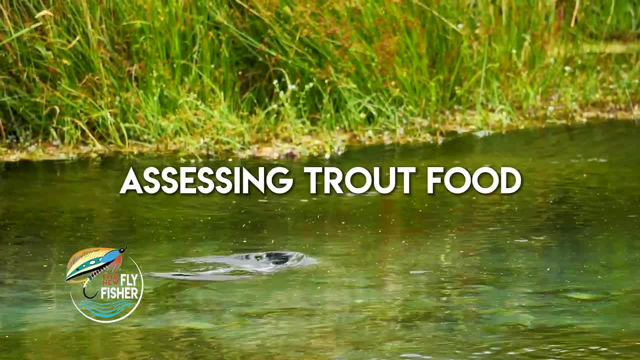 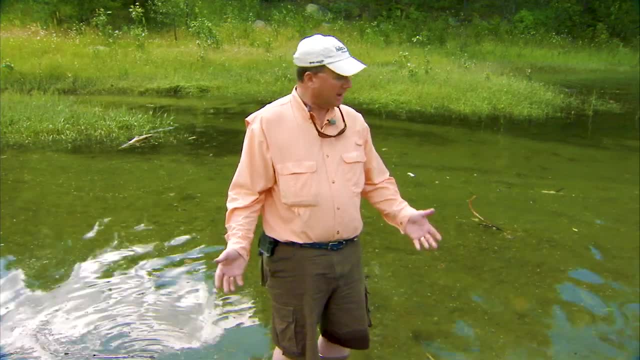 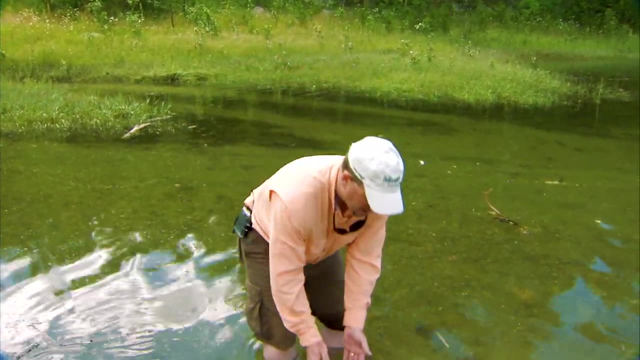 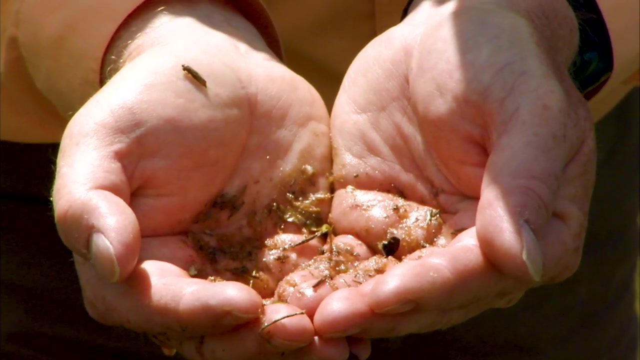 Anytime you go fly fishing, it's always important to pay attention to what's going on around you, And looking around here there is just tons of clues. We've got caddis everywhere around me, So if I take my hands and I'm just going to scoop down, I can see cast pupil, shucks, spent adults, egg layers, adult caddis, themselves still moving around. 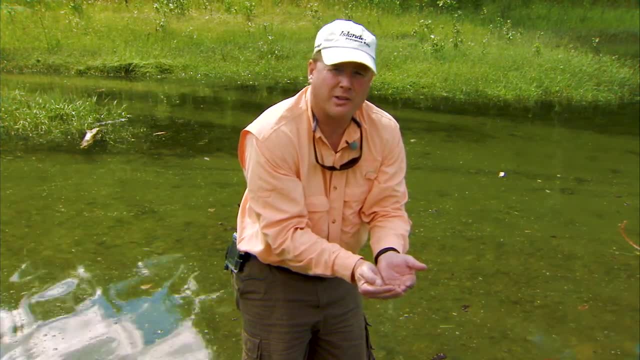 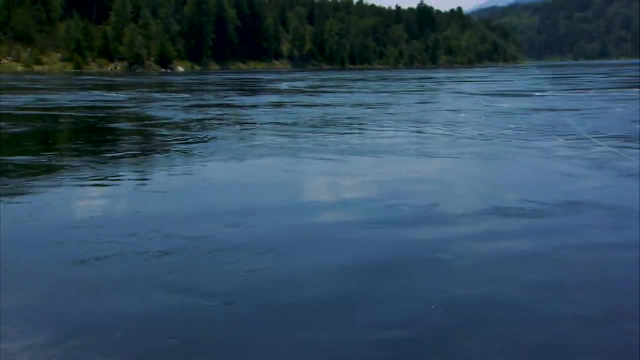 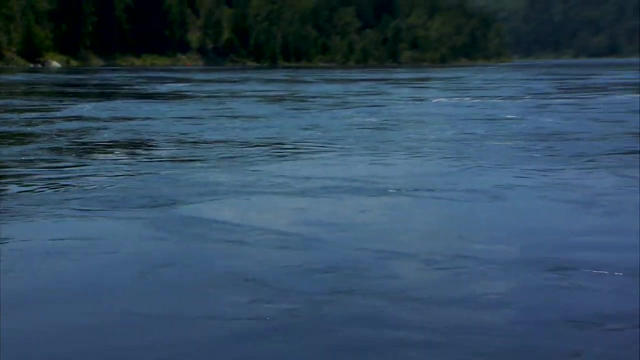 We've got lots of things to think about here today on the Columbia River. Lots of caddis activity- Should be some good, good fishing Coming around the turn. Got to hold this here. let that water come to us. That's good. Here they come, There you go, There we go- Fish on. 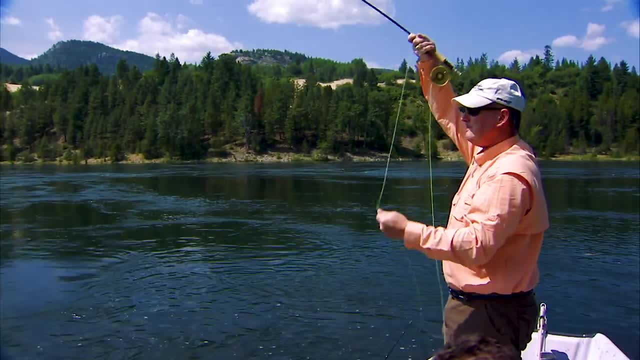 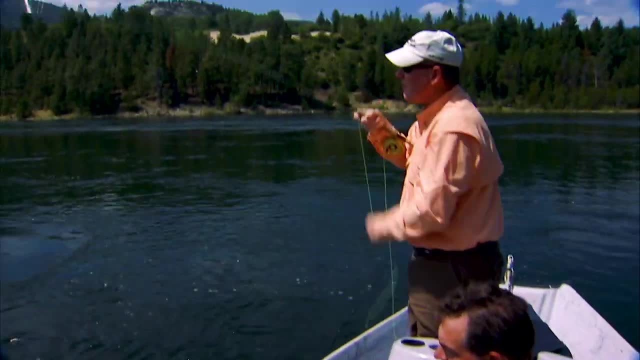 Again that delicate sip, This fish in size 14, antron caddis, I guess you call it, eh Dwayne, That's right, And just a delicate sip, And I'm kind of using my Fly line- is a strike indicator because in all the swirls it's not always easy to pick up the fly. 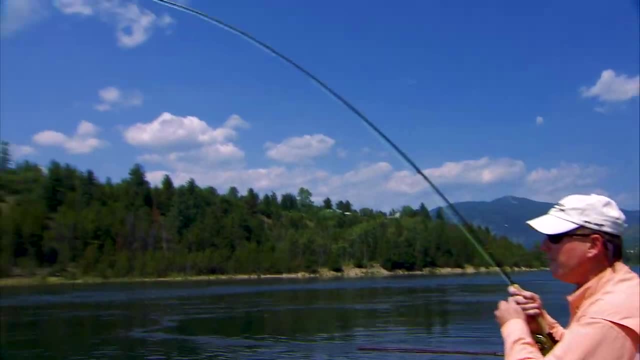 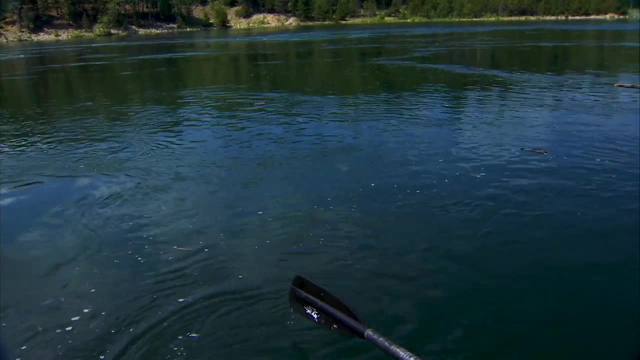 And just saw that little poke and just a gentle lift And lo and behold, I'm connected into a beautiful Columbia River rainbow here. Good for you. Oh, look at this. Look at the color on this fish. This thing is like a hubcap. 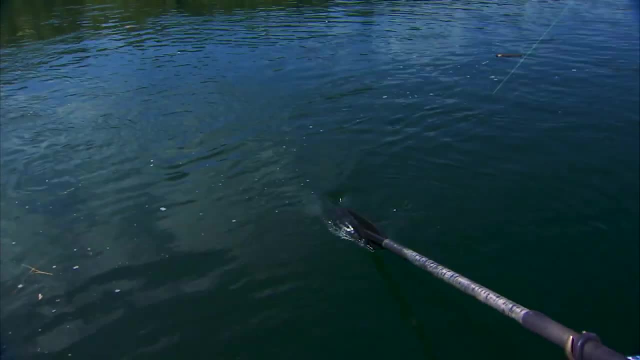 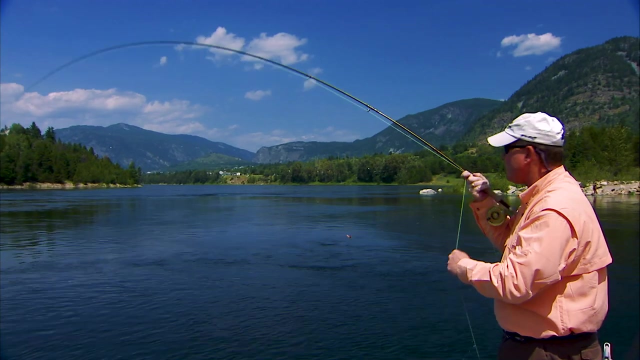 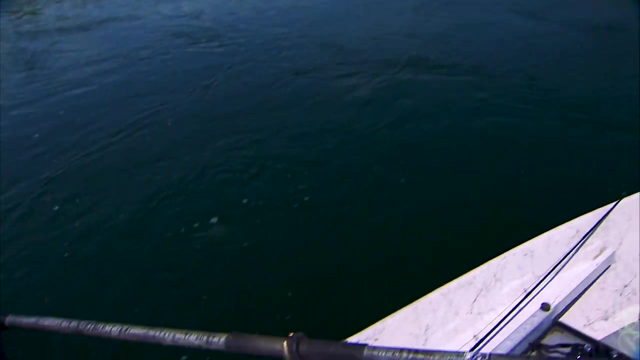 Oh, now it's deciding to go down And these fish can sound. Dwayne was telling us that some of these big, huge Back eddies that we're fishing here, 100 feet deep, That's right Underneath the boat. there it comes up into view. Oh, what a gorgeous, Holy smokes, what a fish. 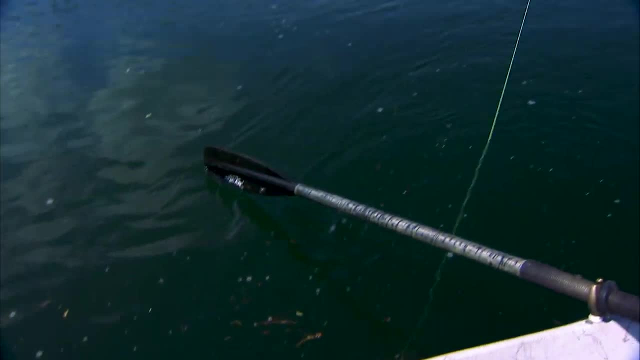 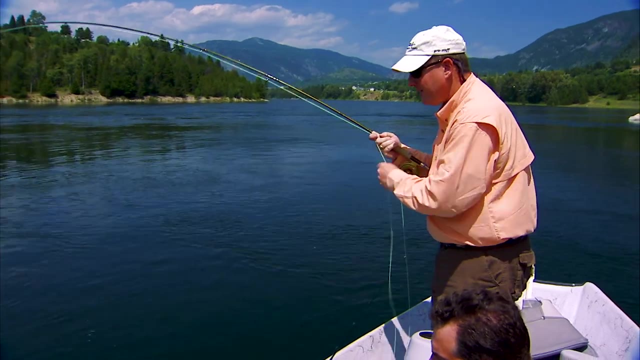 Yeah, they usually run a few times. Oh yeah, He's figured that out. Yeah, Three times, and then we'll be able to net them. Yeah, this guy didn't. He's kind of confined himself into the flat water here, which works to our advantage. 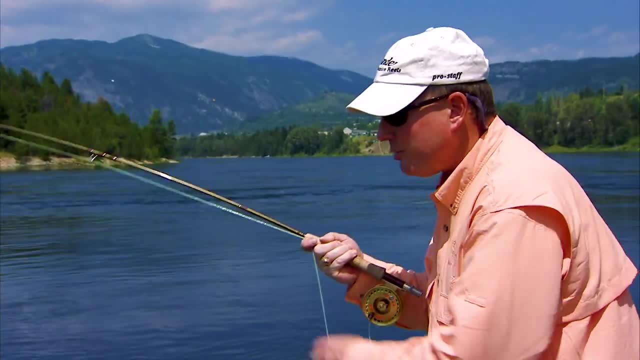 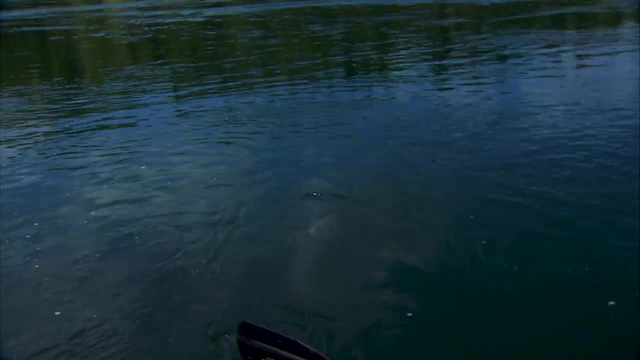 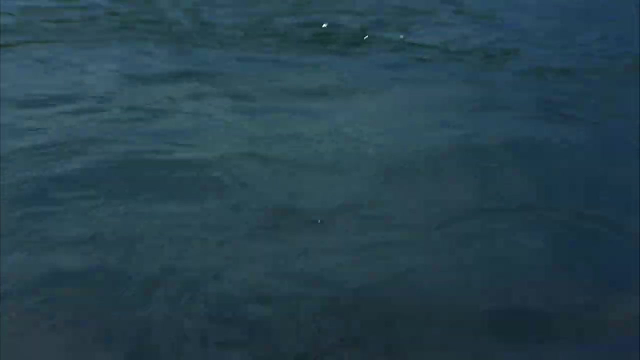 That first one, I had hit the main current and adios backing: Oh, this is a gorgeous fish, Holy smokes, Holy smokes. This is the stuff, I'll be honest, I'm used to seeing in lakes. Yeah, Might be an idea to do a little line management here.